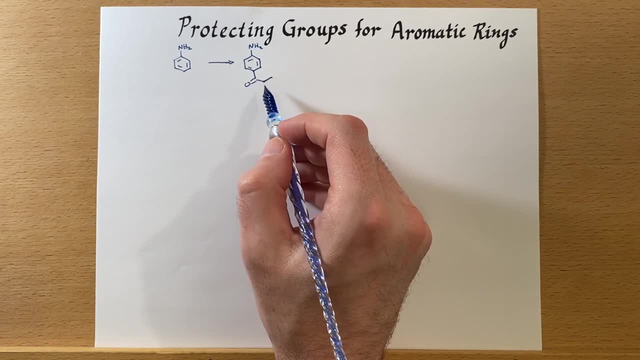 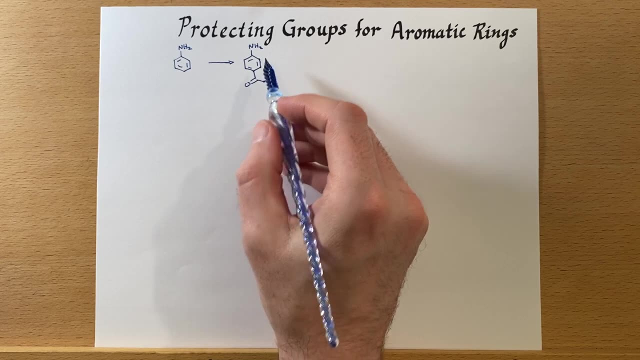 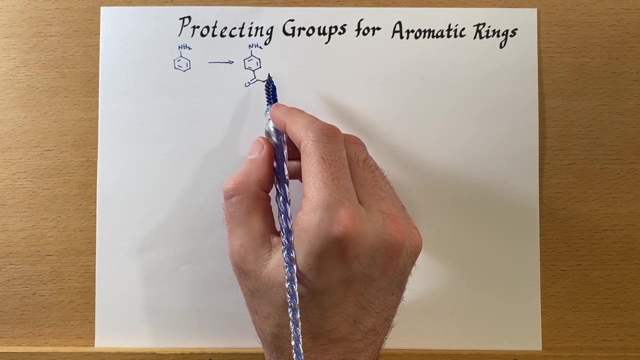 molecule. right here The problem is we can't directly add the nitrogen to the aniline, but we can add this on with the nitrogen exposed. This is a Lewis base and in order for this reaction to take place, we would need a Lewis acid catalyst And the reaction that we would 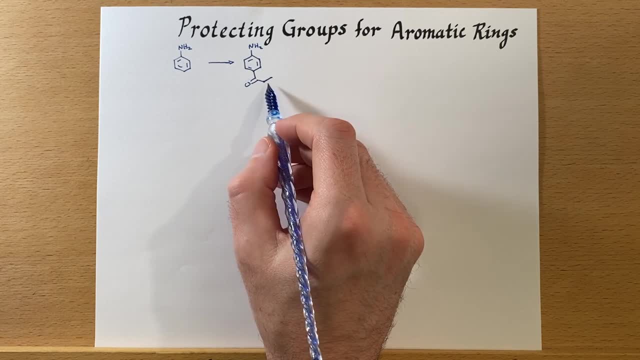 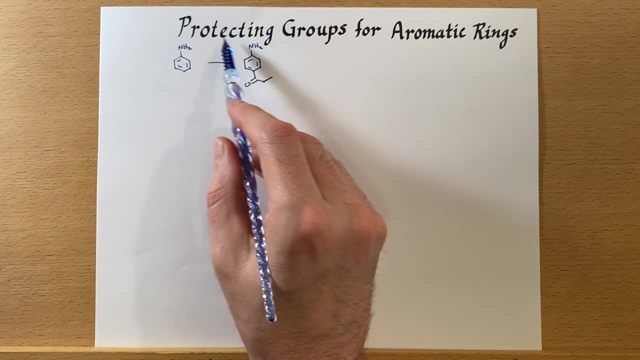 want to have happen is this: Friedel-Crafts acylation. What will actually happen is that our aniline is going to be in the right direction and we're going to need a Lewis acid catalyst And we're going to need a Lewis acid catalyst, And the reaction that we would want to have happen is this: Friedel-Crafts acylation. 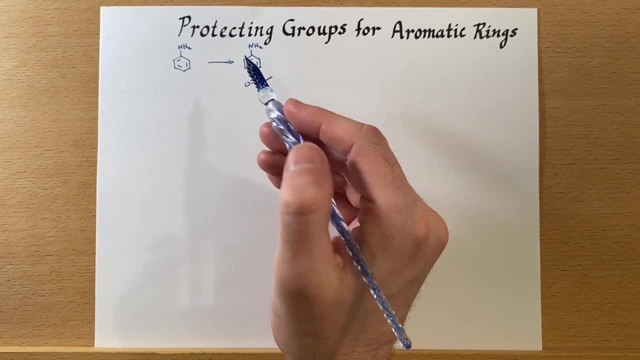 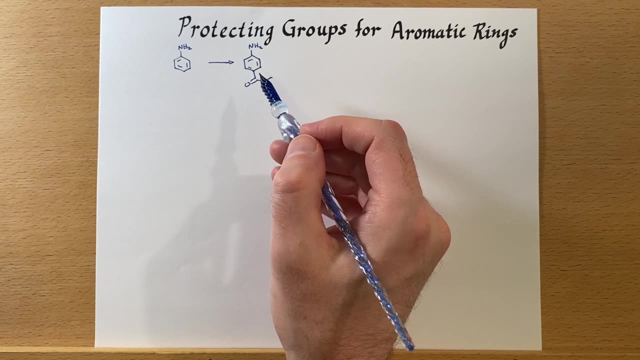 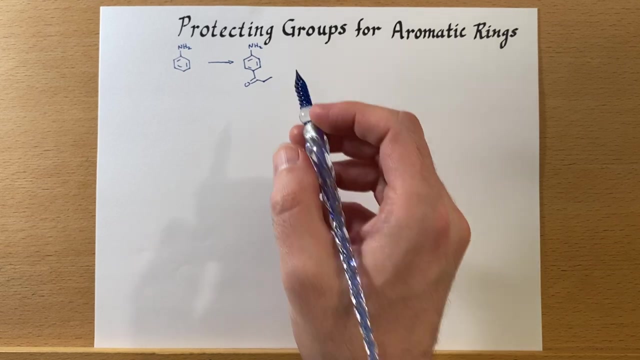 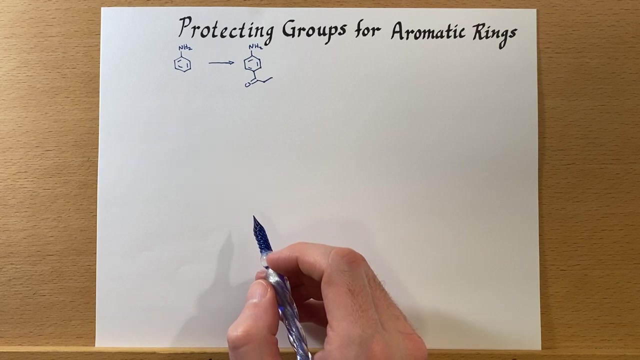 going to react with our catalyst, our Lewis acid catalyst, and destroy it, And so we can't go directly without covering up this group right here. So somehow we must protect the amine Now. a while back we've talked about amides, And amides have these same directing. 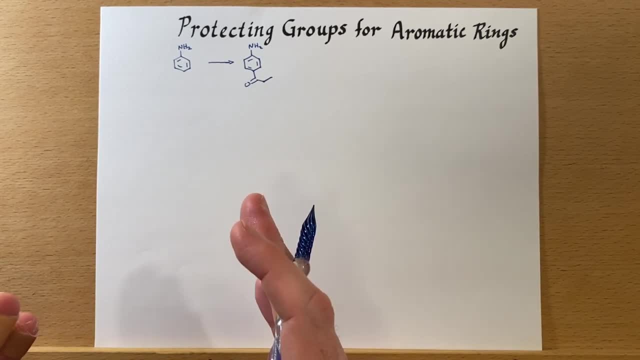 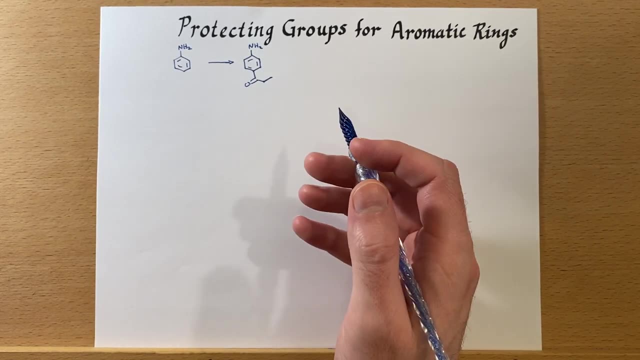 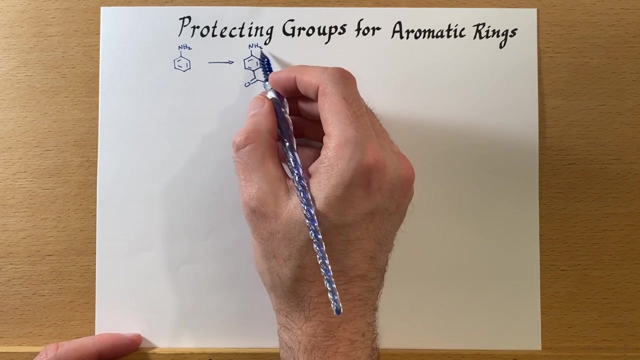 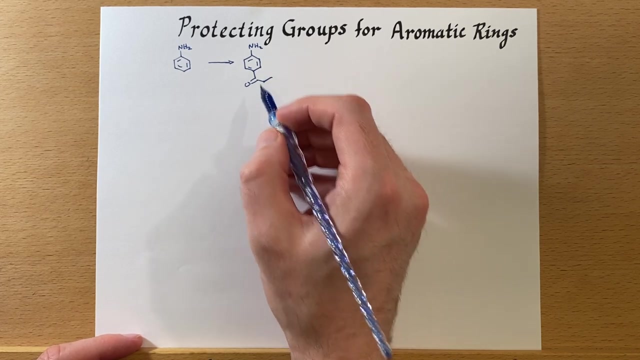 group right that they direct ortho para as well. as same as the nitrogens, just the amine. But amides are much less reactive. So what we can do is convert this amine into an amide. That will vastly reduce its reactivity. Then we can come in and acylate. 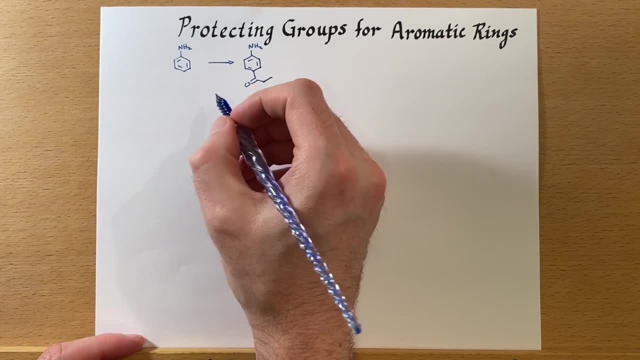 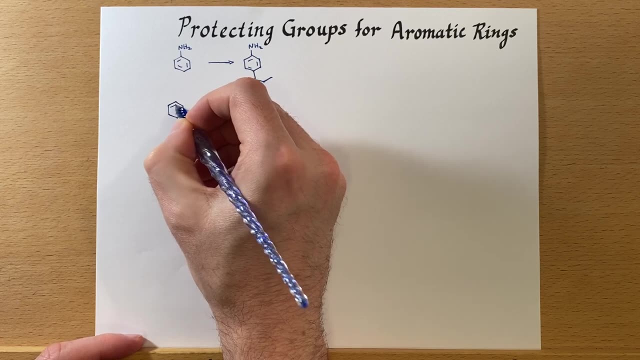 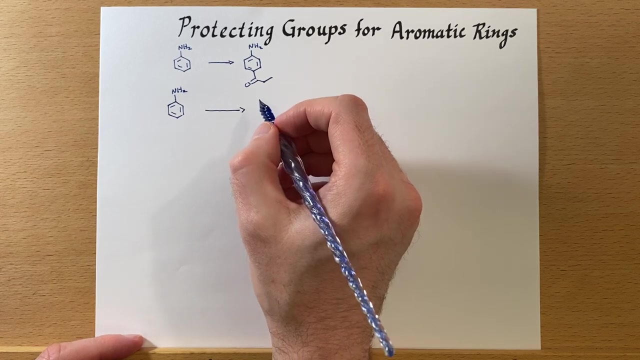 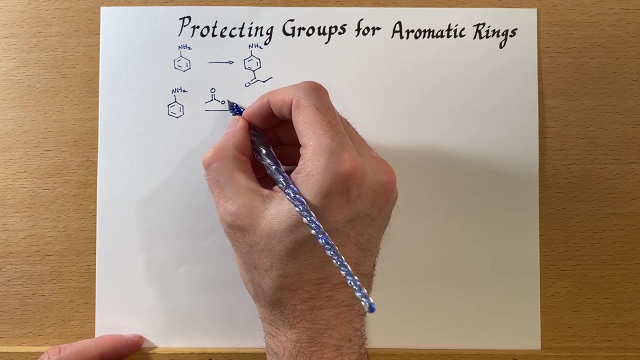 And then we can hydrolyze amide. So let's look at this process. So, beginning with aniline, we form an amide. Now we could use either an acid chloride or an acid anhydride, So we'll just use. 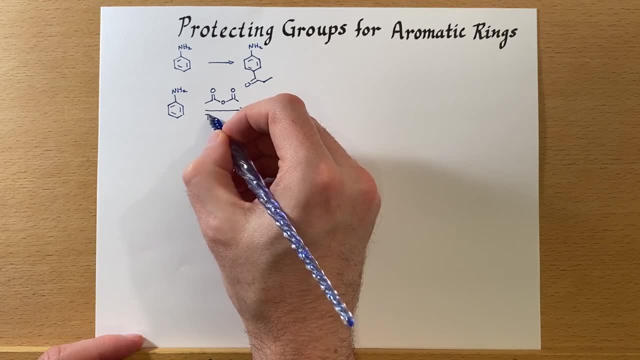 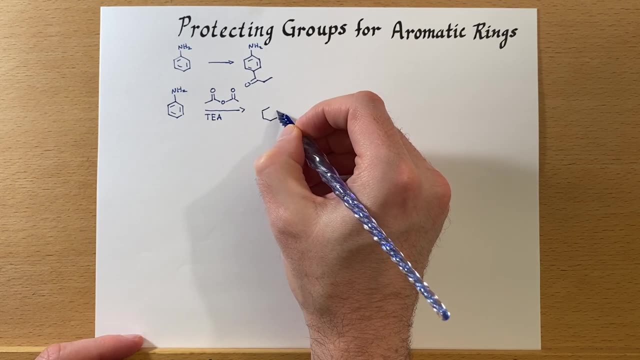 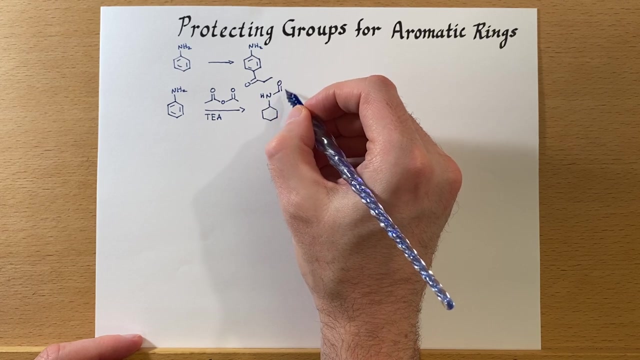 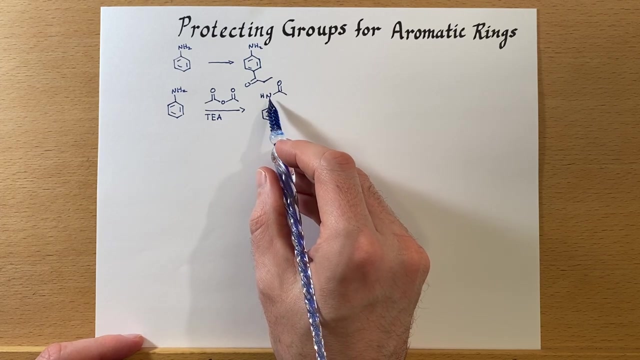 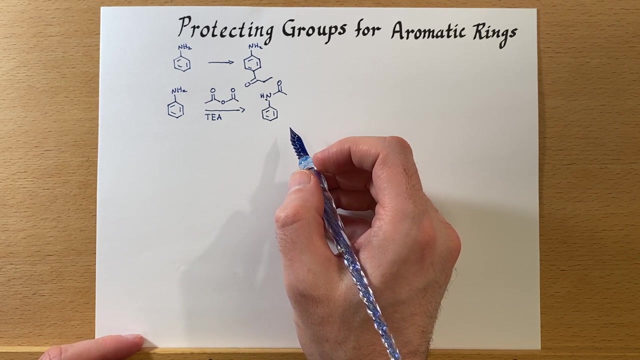 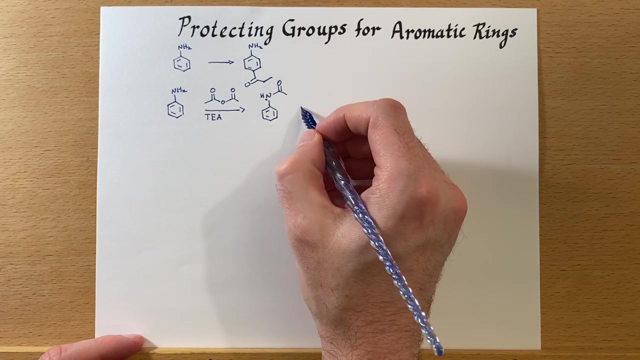 acetic anhydride here and we'll need some base like triethylamine. Next we will form the amide. Now this is still activating because we still have a lone pair on that nitrogen and it is still ortho-para-directing. But amides are much less reactive than amines. So now we 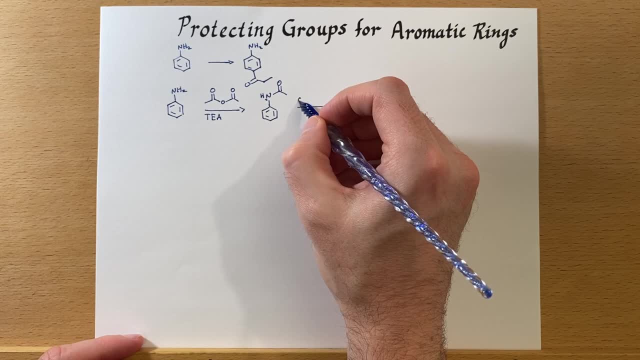 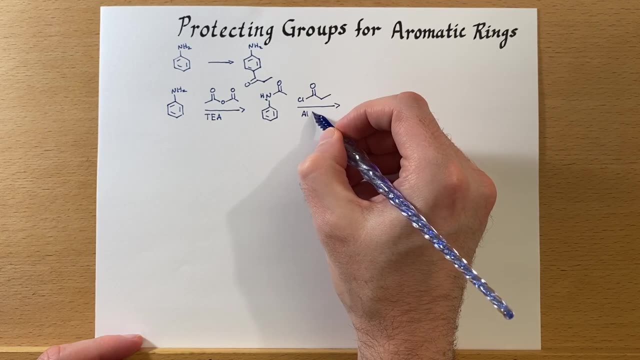 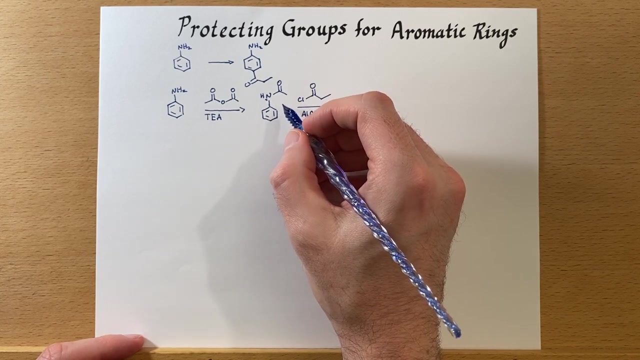 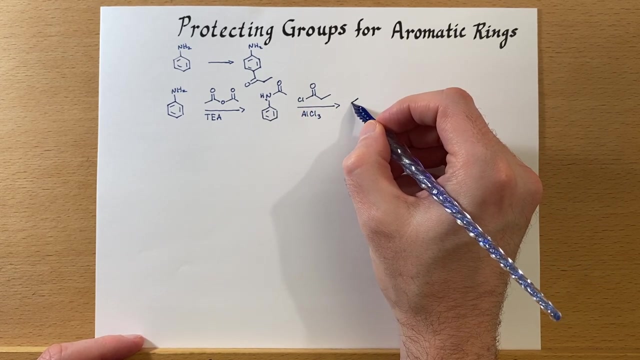 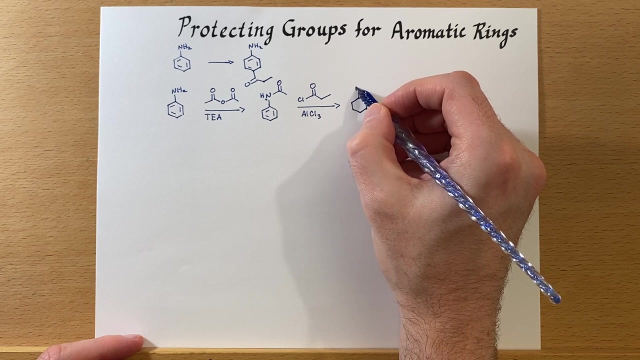 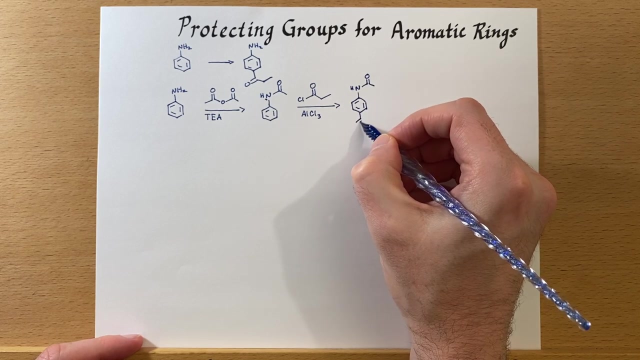 can carry out the acylation without difficulty, And this is a bulkier group too. So it's going to kind of block the ortho positions a little bit, and that will help guide it towards the para position, which is what we were targeting anyway. Next we'll just 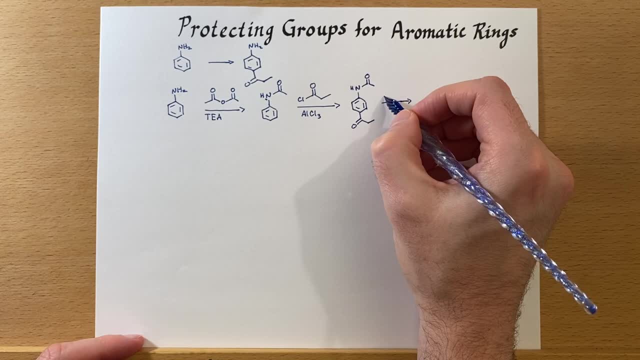 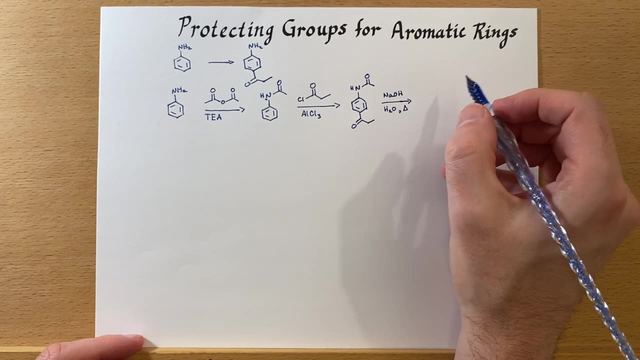 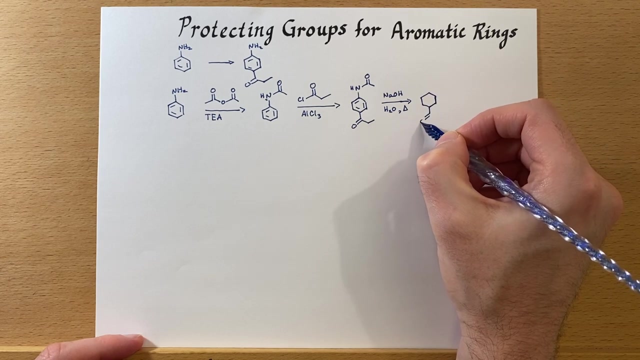 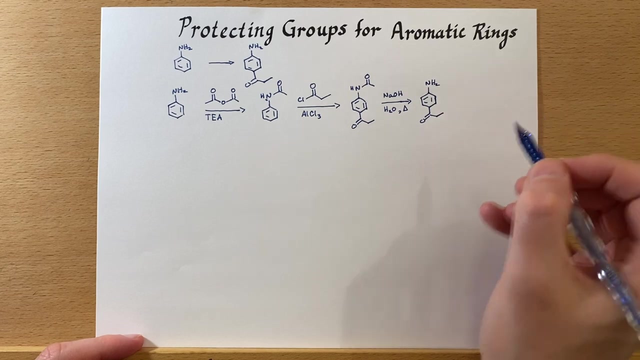 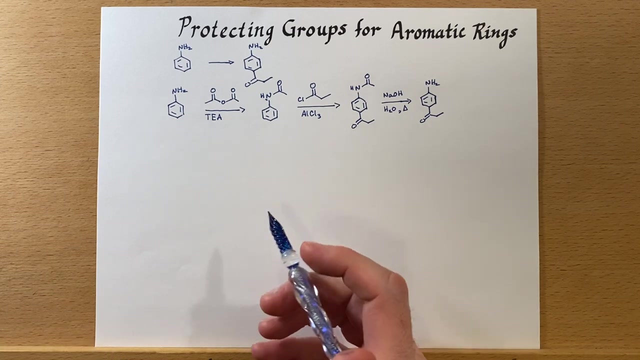 hydrolyze the amide. So we're going to take theplat anhydride and we're going to. so that's one potential for protecting something on an aromatic ring. Now let's look at the number of petals. Next, we're going to take our basal platelet. We're going to 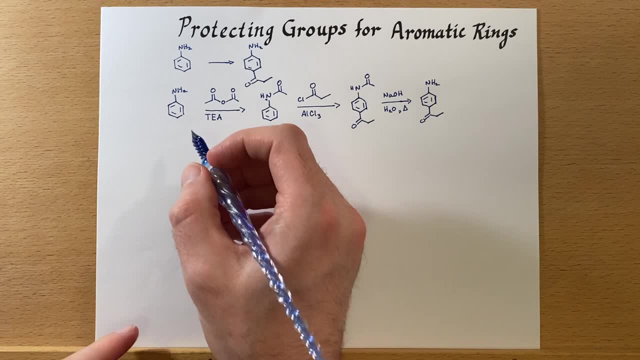 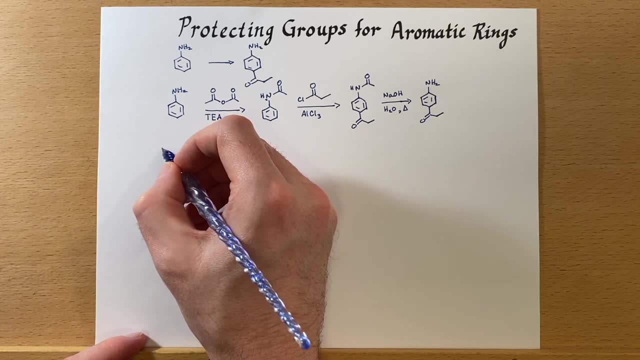 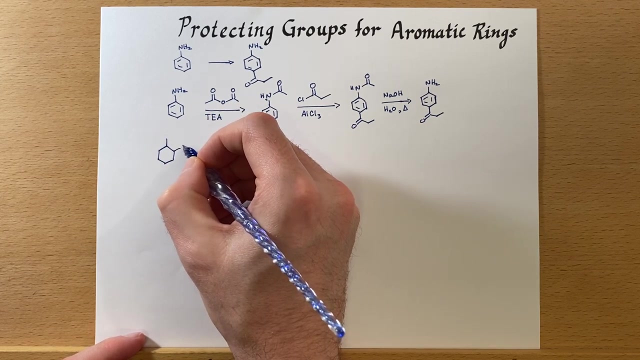 put this on the top of the amide and we're going to place a small part of this. another reaction that we may want to do. let's target the ortho isomer or the ortho position on this phenol. so we would like a bromine. 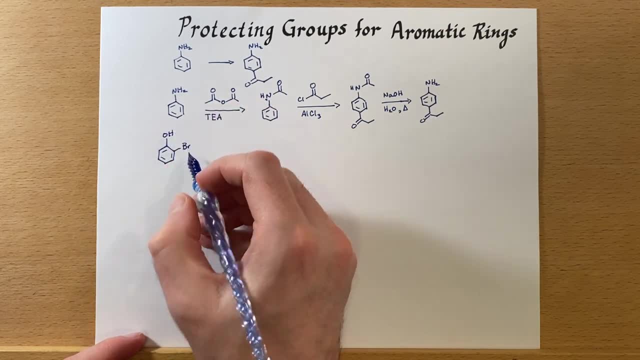 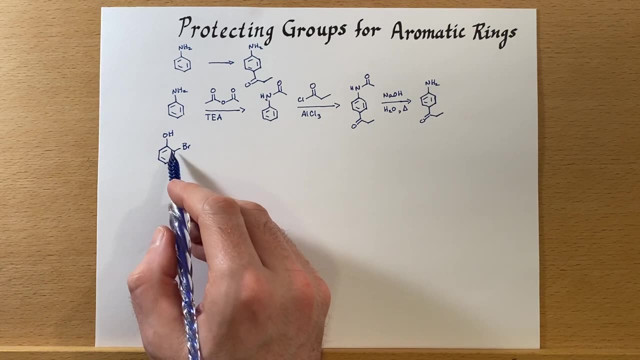 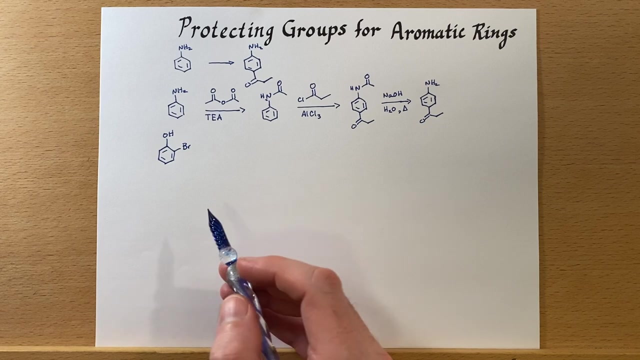 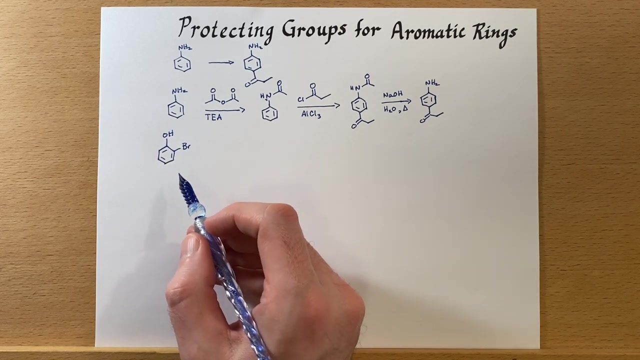 to end up ortho to the phenol and if we just ran this reaction and said: all right, we've got phenol, we're going to add bromine and we can even do this without adding the iron catalyst. we probably should, because this is an activated ring and if we added the iron catalyst we may over brominate. 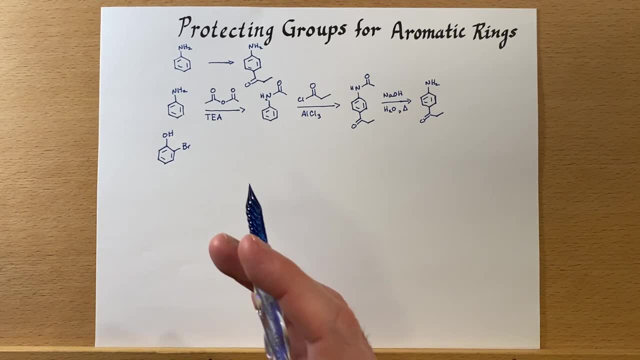 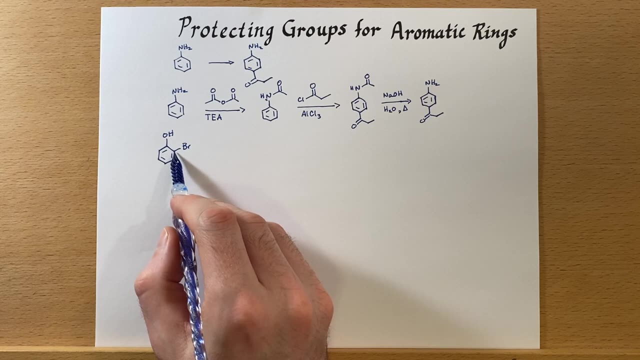 the ring you. that's not necessarily the problem we're going to deal with right now. the second problem is that there's nothing stopping it from attaching in the para position. well, we want the ortho position to be substituted. so what? what can we do? well, if, if we had some group here in the para position, we could stop it from. 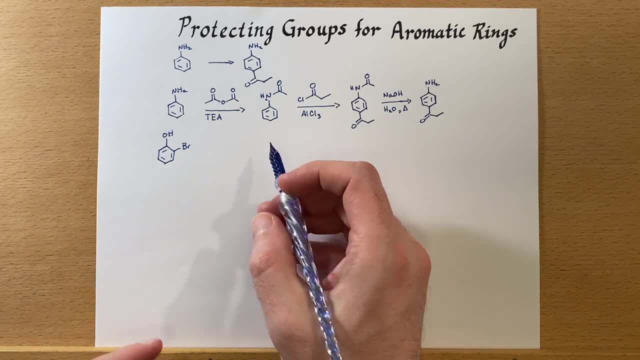 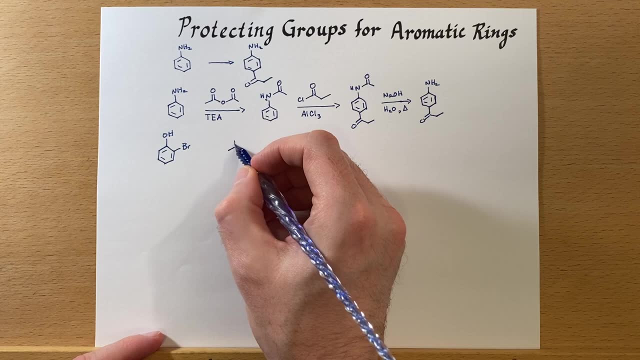 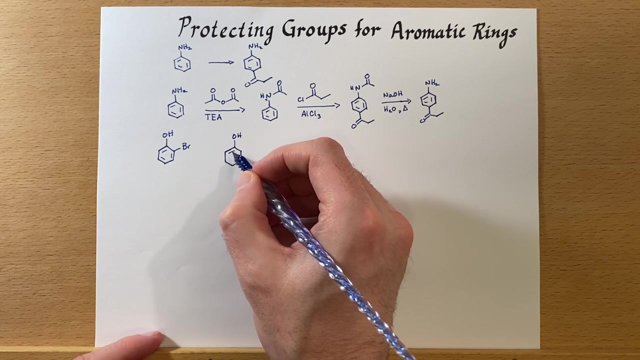 reaching the ortho position and we could stop it from attaching in the para position reacting because it's already occupied. so we do have a reagent that will do that. we could sulfonate this now. if you recall, sulfonation reactions are reversible and that's kind of important. 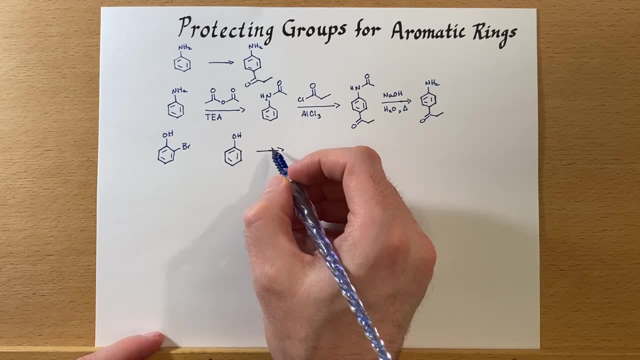 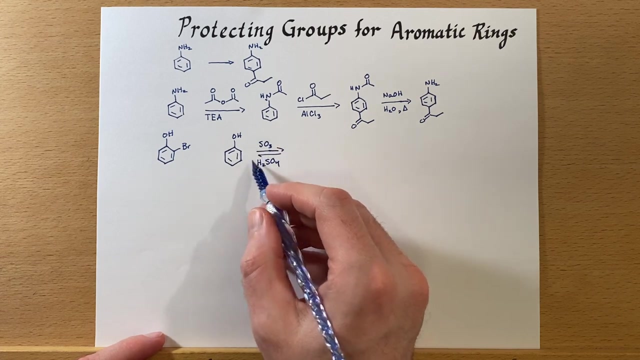 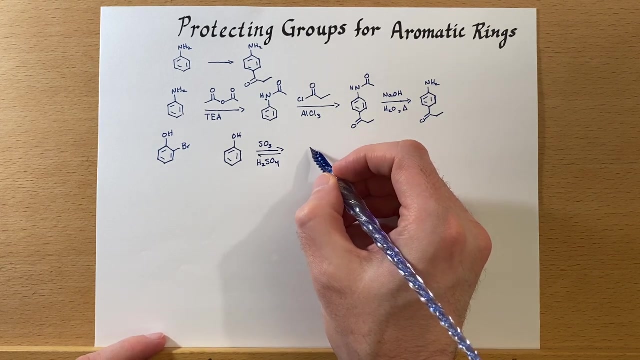 if we're considering this to be a protecting group. so we need fuming uh sulfuric acid. so this is one way to write fuming sulfuric acid. we have so3 crammed into concentrated sulfuric acid and this will preferentially add to the para position. 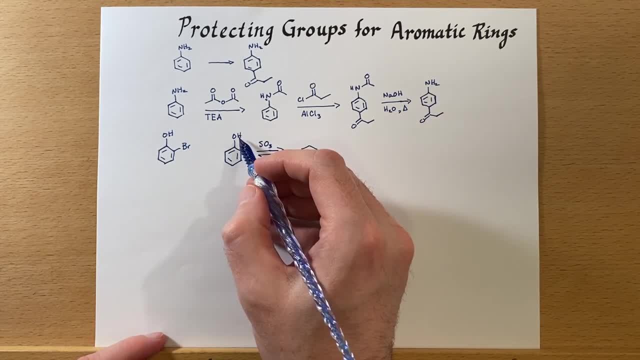 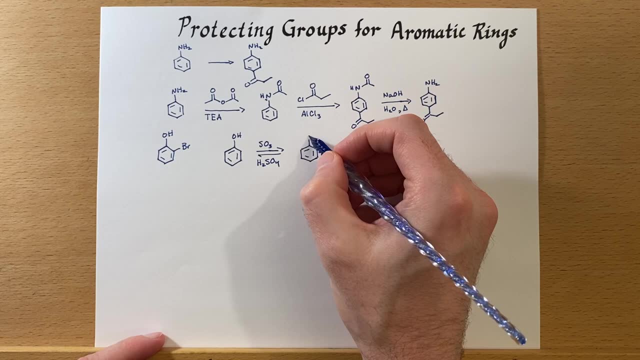 now, this is an ortho para director, so it could it could have gone here or it could go in the para position. the reason why it preferentially goes in the para position is because it's not the para position is. this is a sterically bulky group. 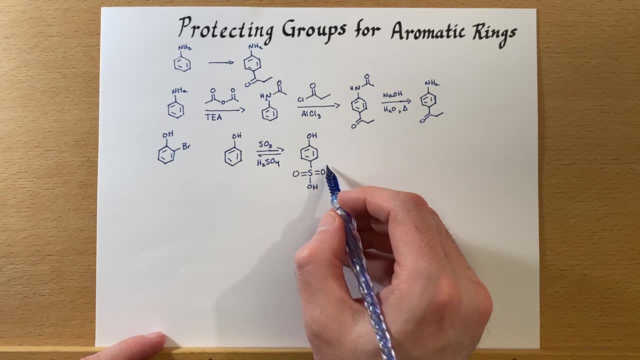 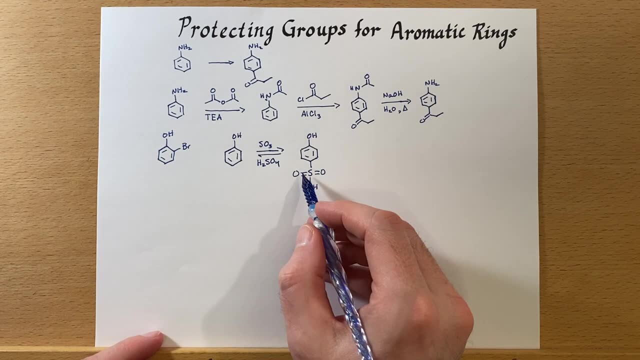 i'm drawing it out this way, so you can kind of see that if i had a group here, ortho to the sulfonate- there would be a little bit of bumping into each other going on. so this preferentially adds into the para position now. 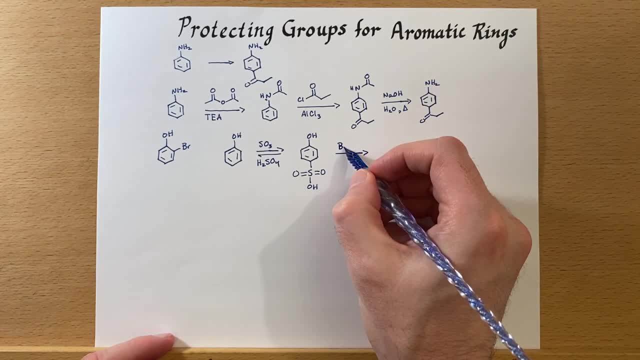 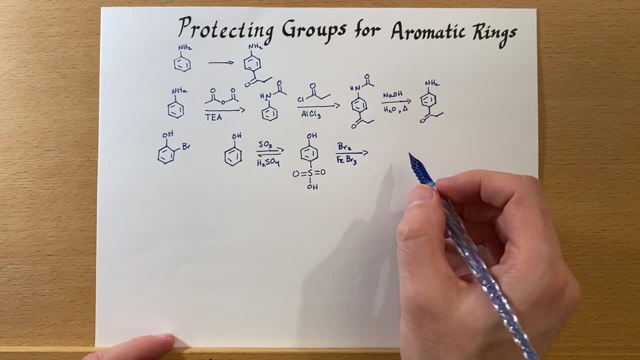 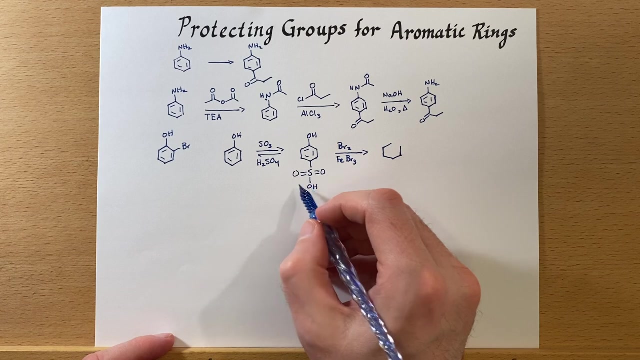 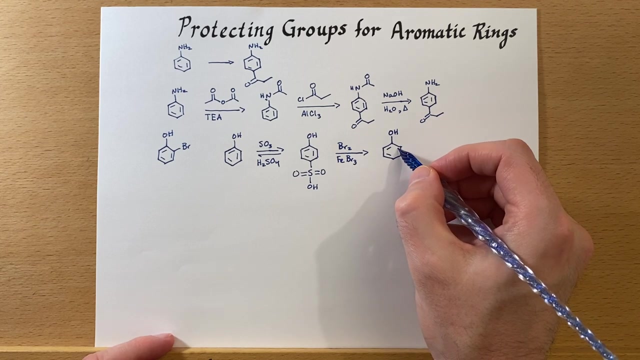 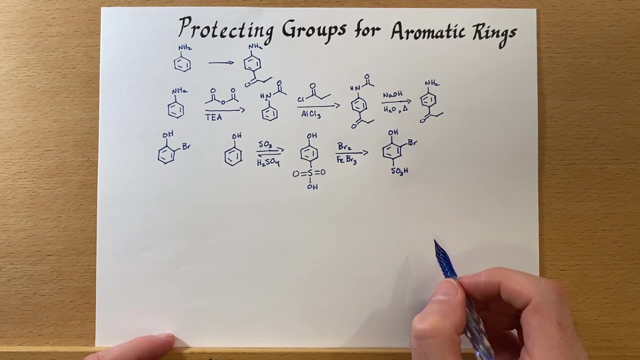 next, we can go ahead and add in our bromine- and we'll probably need the catalyst here, because this is a little bit electron drawing, so A little bit deactivating- And now that the para position is blocked, we can substitute in the ortho position. 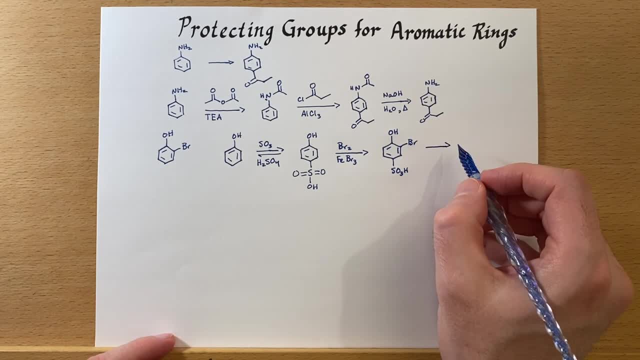 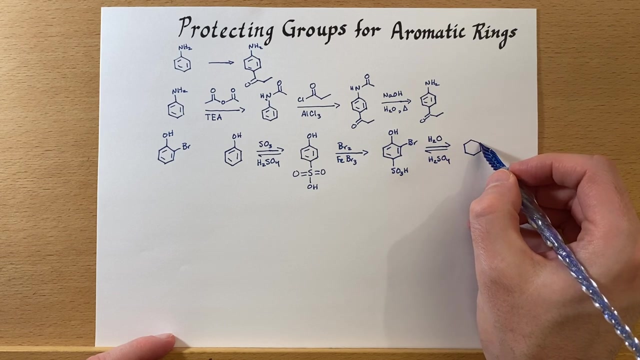 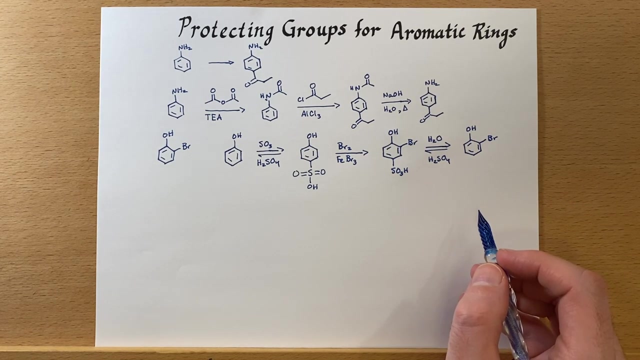 And then, as all good protecting groups are, we can remove it using some water and a little bit of sulfuric acid, And now we have generated the ortho isomer without worry of having to make a lot of the para isomer, And of course this was really advantageous that sulfonation is reversible. 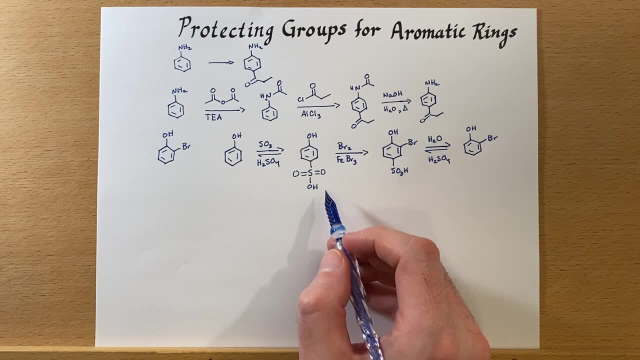 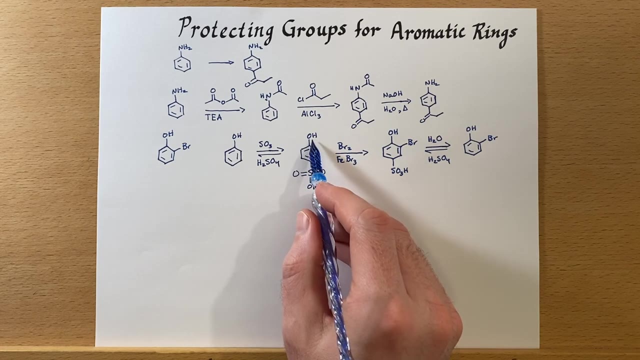 And considering that this is a deactivating group, we don't really change where on the ring this will end up, But since it's deactivating, it will be a meta director. So meta to it is also ortho to this ortho director. 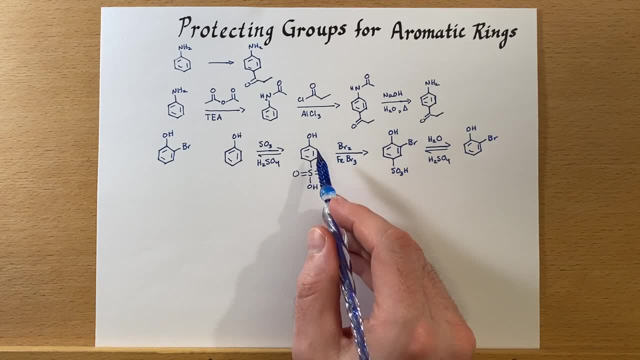 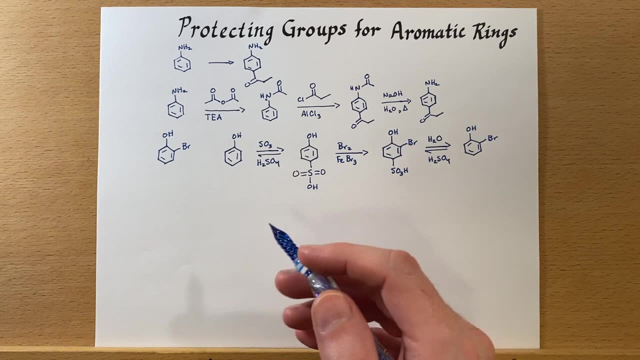 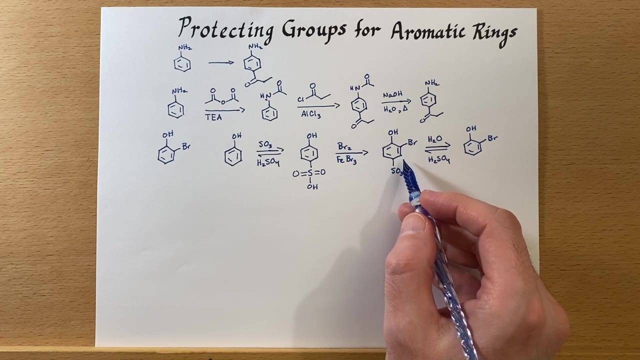 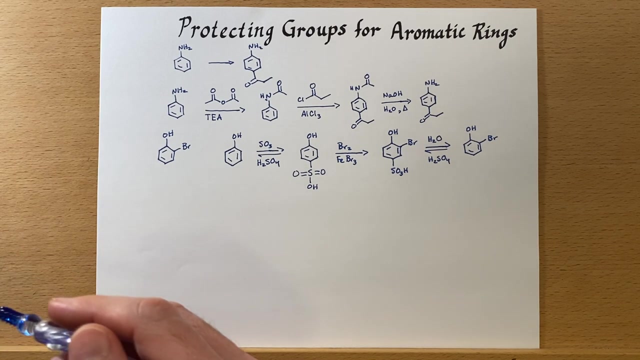 But since the alcohol is an activating group, it will take preference anyway. So I guess that's a lot of ways to say this is a way to guarantee that you'll make the ortho isomer rather than the para one. Let's look at another possibility of transformations. 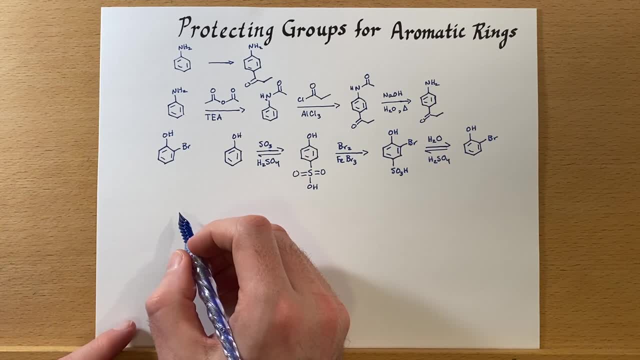 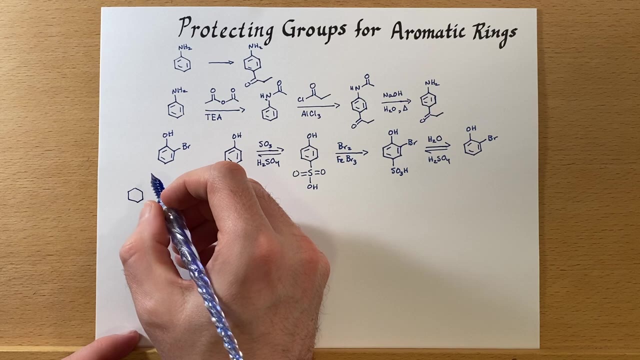 And we're going to try to take para Okay. Okay, So we're going to take para methyl aniline and turn it into meta chloro toluene. So I'll just draw up what we're doing up here and then you'll see like that is quite a bunch. 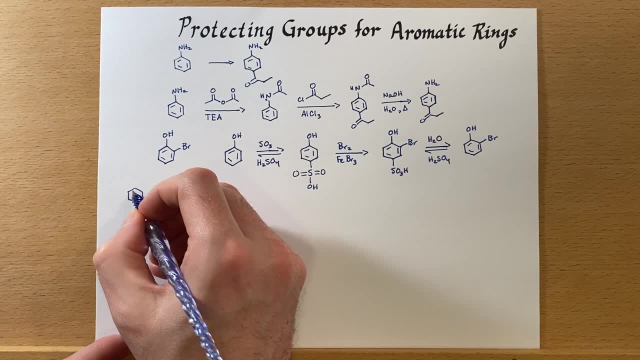 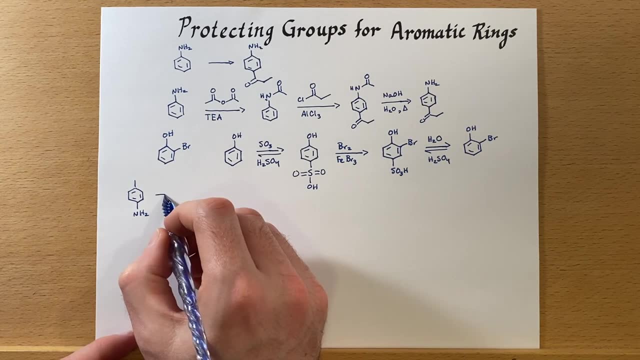 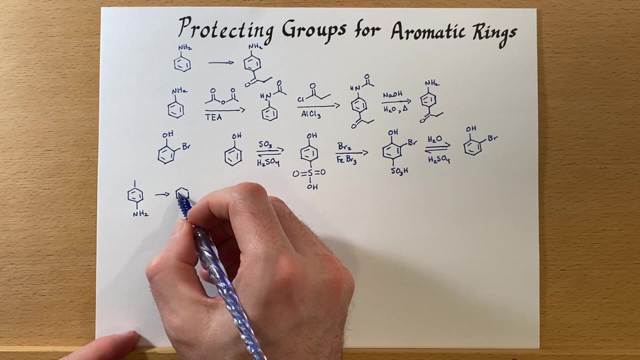 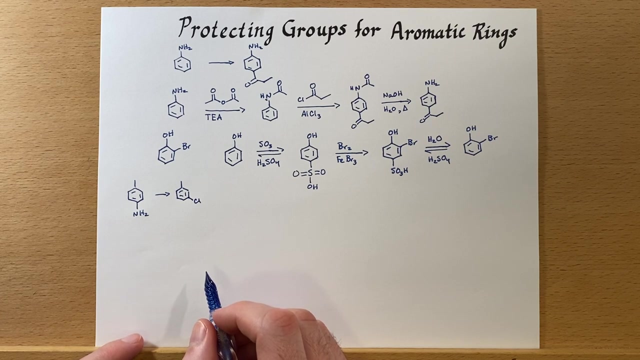 of reactions here. So we have para methyl aniline And we would like to turn this into Meta chloro toluene. So here's toluene and then chloro right there. So let's see what we can do. Well, this is an ortho para direct. 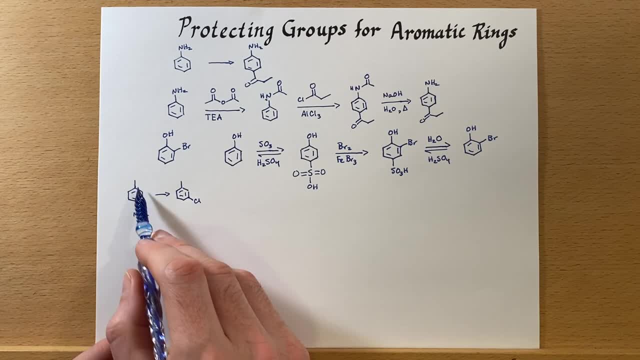 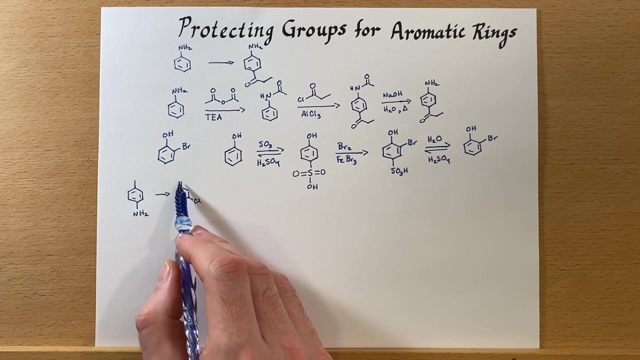 Okay, So this is an ortho para direct. Okay, So if we try to do this directly, we may have a little bit of a problem getting it to go into this position right, Because some of it will also end up next to the methyl group up here. 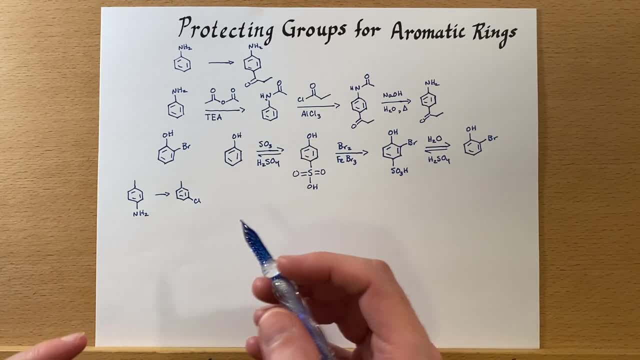 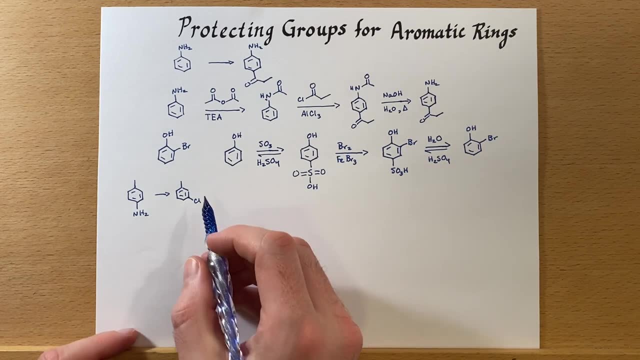 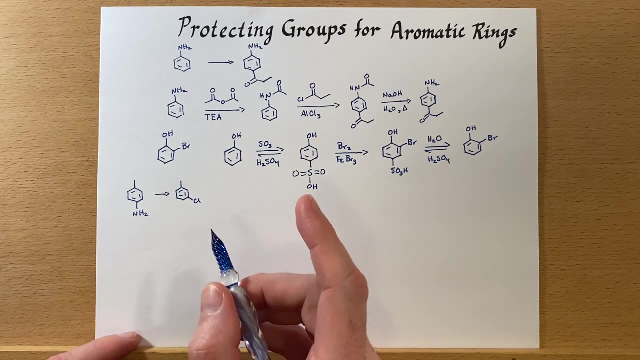 So, and we may actually over chlorinate, Okay. Okay, Because both of these are activating, And maybe that's the bigger problem actually. So we're going to start off by lowering the ring activation. So we're going to do the same thing that we did up here. 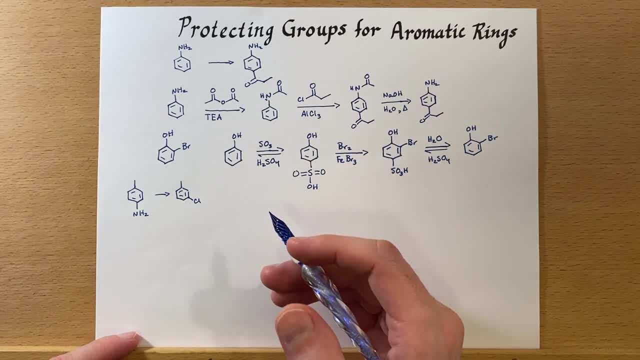 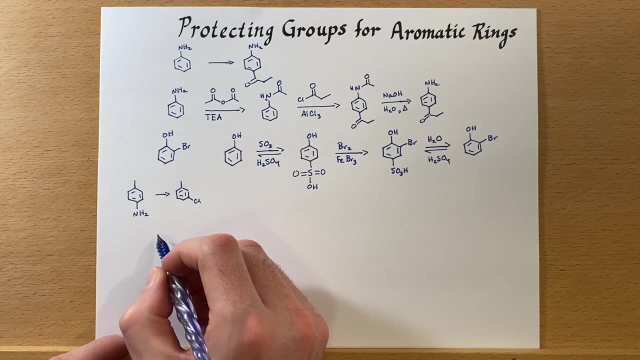 We'll form an amide that will slightly deactivate the ring. Then we will not over chlorinate. Okay, Okay, Okay, Okay, Okay, All right, So we do that, And I'm just going to start from here and start drawing my reaction there. 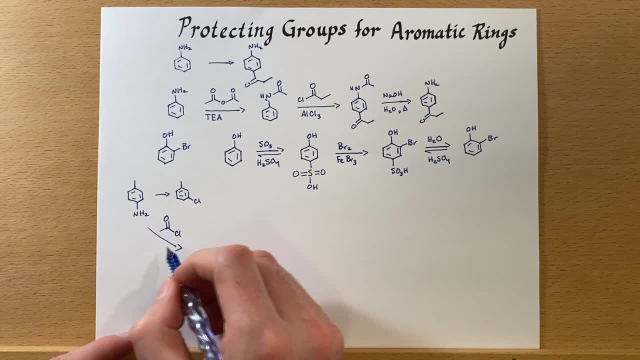 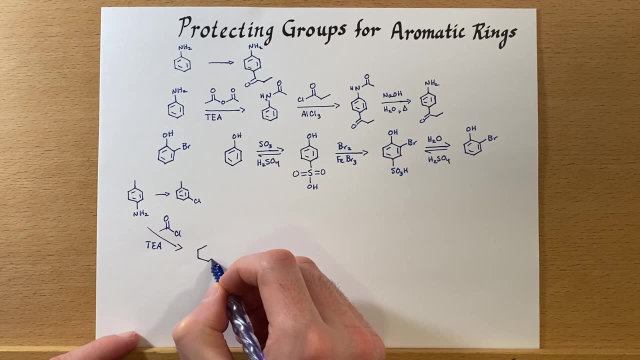 This time I'll show you Rusing the acid chloride to do the protection. We're going to do it clearly. Five seconds, One now. we have that now. we do not wish to over chlorinate, so we're not going to add in any. 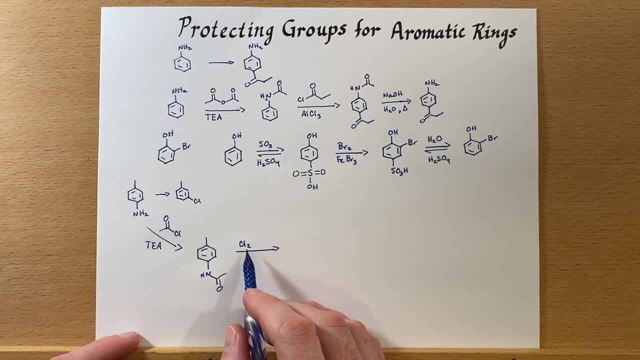 of our catalyst and when we do this we will be able to ortho direct right here, because the this is not as strong of a directing group as the amid is. it's got lone pairs. it can really donate things in lots of resonance structures that we can do. 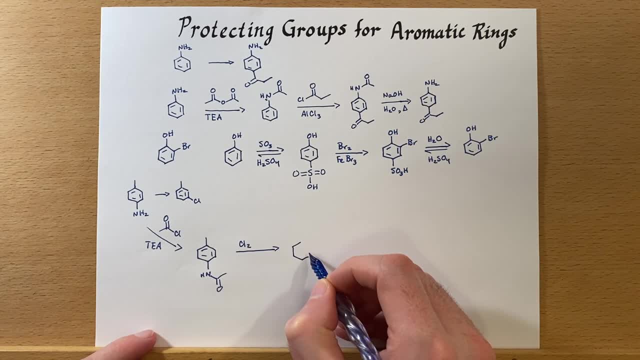 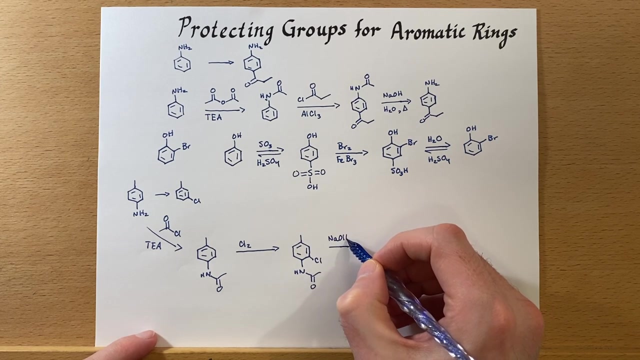 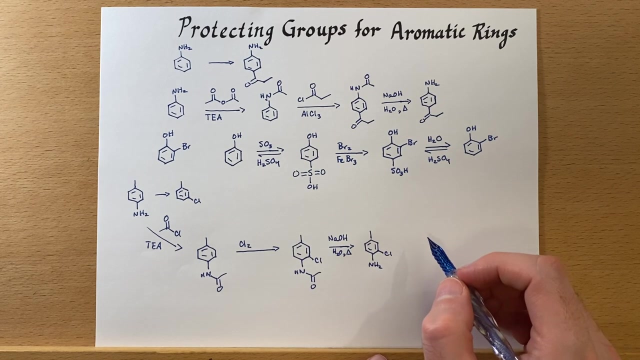 you. so now we've made this and at this point we're getting close to our target. we just need to remove this. so first we'll remove the protecting group, that amid. that will make this a little bit more reactive. so we go back to the amine and now we're going to form the benzodiazepine. 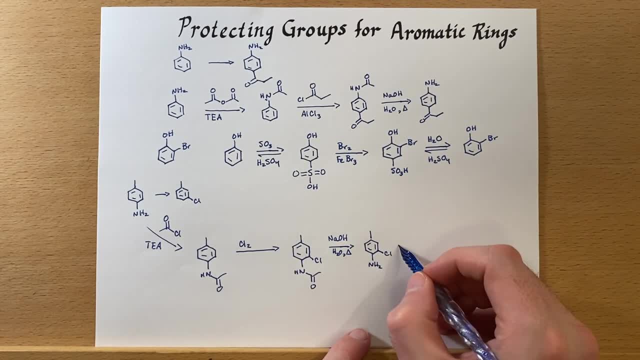 brigade. at that point we made it by adding a tiny bit of holders. it's a turning body that is running in a straight line. and now we're city. we're going to form the welded trillion hydrochlorates block governor. claire, we're just going to get loose. 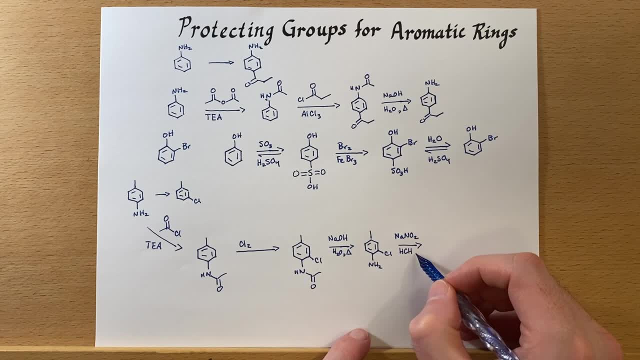 everything and to give it just a bit more freshness, we're going to take one cup of our bottles here, look at this and then- and we're going to let it rest for a little bit of time, and then we just use one of those Sandmeyer reactions to remove these. 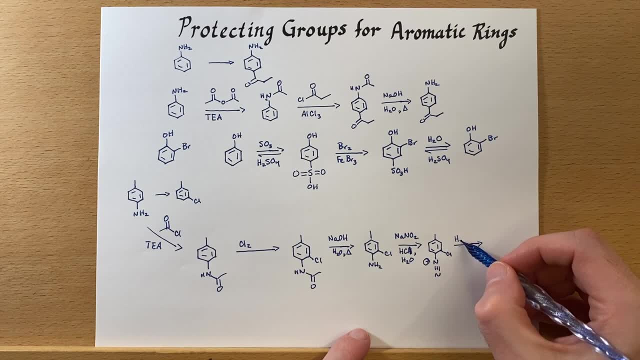 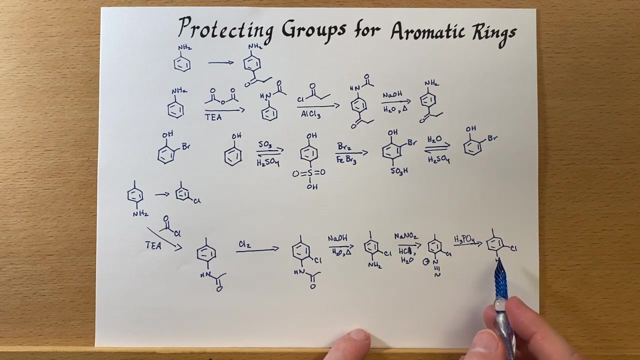 nitrogens. So if we add phosphoric acid in here, then we'll remove this and replace it with a proton, And now we've completed the synthesis without over chlorinating and in the correct position. So that's a little bit on protecting groups for. 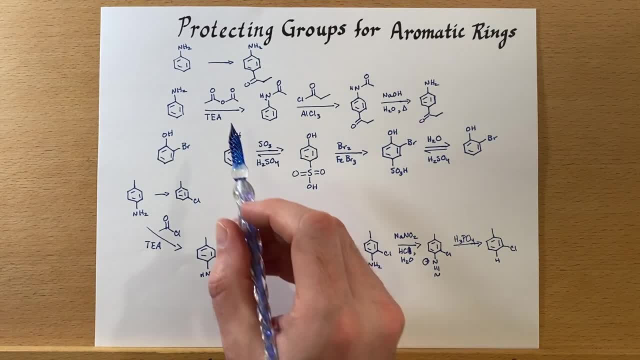 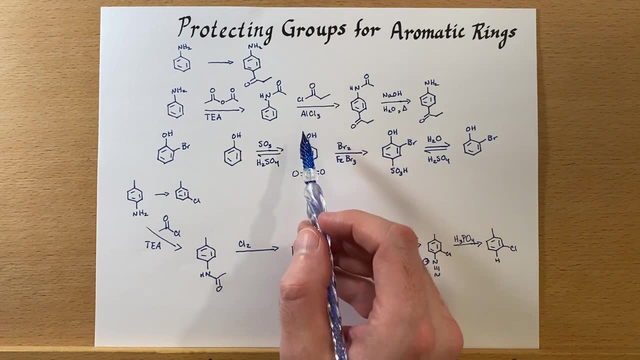 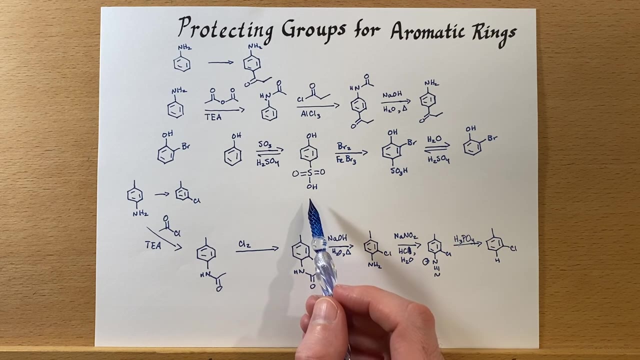 aromatic rings. Sometimes we'll need to protect an amine or something that could react with our catalysts, And sometimes we're looking to block a particular position on a ring, such as the para position. It's not as important to block a position when we're looking at meta directors, because